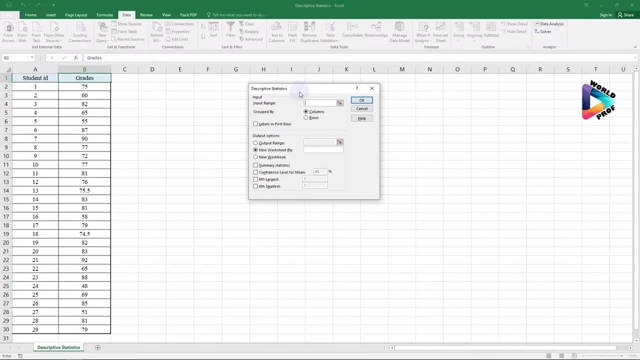 OK, now the first thing that we need to enter is our input range. our input range is the data we want to analyze. so here, in my case, I have student grades, so I'm gonna select all values in the column. so, because I also selected the name of the column, 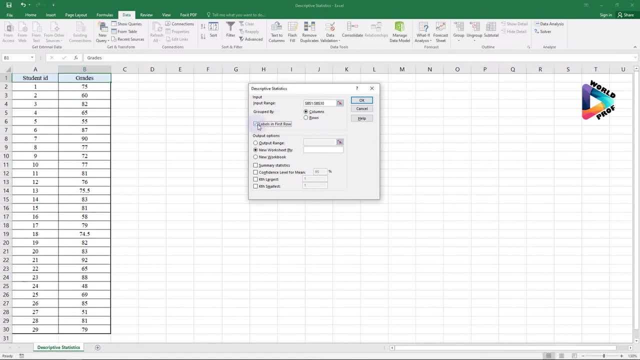 here the header. so I need to check this box labels in first row. and then you need to make sure that summary statistics and confidence level for mean and ninety-five percent are checked. and here you see, you have three elements that you need to check. and here you see you have three elements that you need to check. and here you see, you have three elements that you need to check. 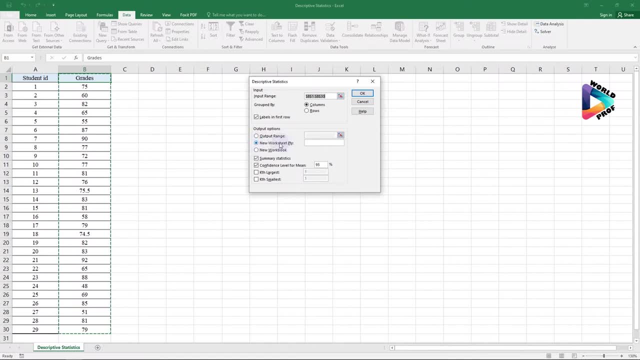 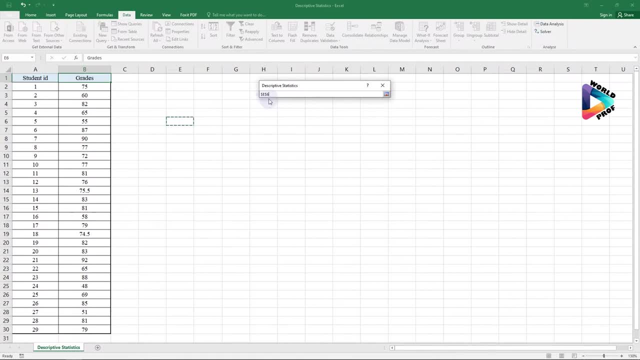 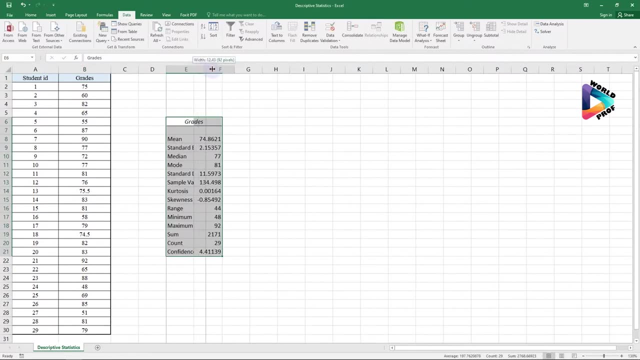 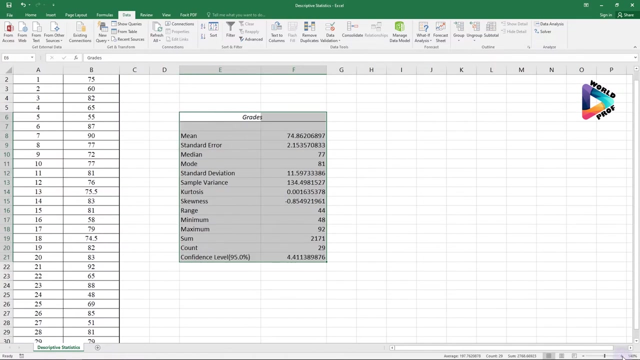 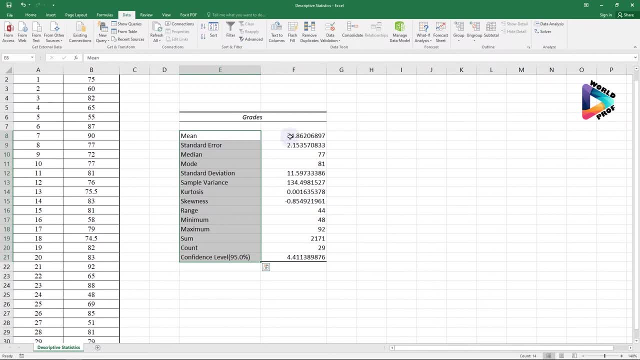 different measures and in front of each measure I have the values. The first one is the mean. The average grade in this class is 74.86.. Then I have the standard error. Sometimes when you look at a standard error you're confused because standard error is similar to standard deviation. but here you need to. 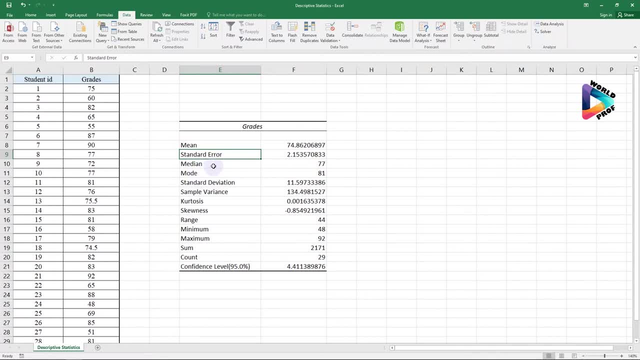 understand that standard error tells us how close our sample mean is to the true mean of the overall population. But the standard deviation? it tells us about the shape of our distribution. It basically tells us how close the individual data values are from the mean value. So that's about standard error and standard. 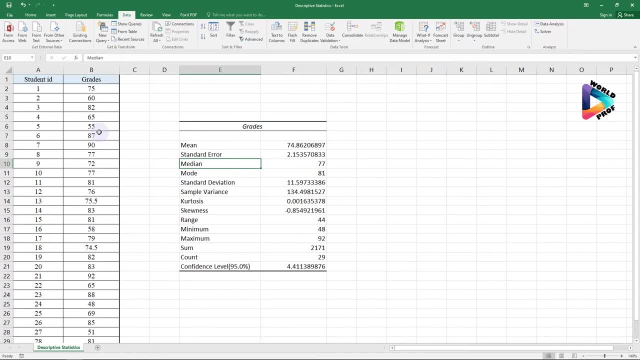 deviation. Then we have the median Median is a number which is in the middle of our data. Okay, so 77 is the number in the middle. And we have mode. So mode is the value that has a higher frequency compared to other numbers that we see in the data set. So here it says. 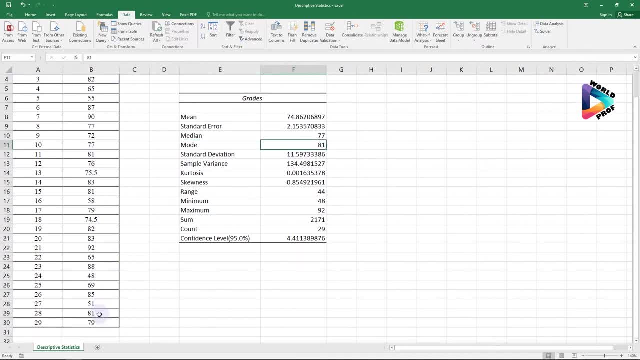 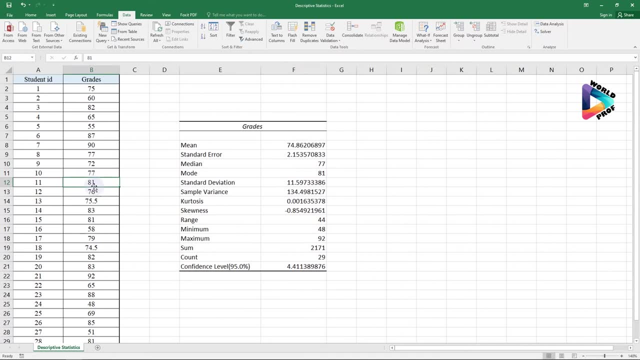 81, and that's true. if you look at the data set, we see that 81 here and 81. So we see 81 a couple of times in our data set. You also see 77, but you see it twice. So 81 has the highest frequency. If you don't see any mode, 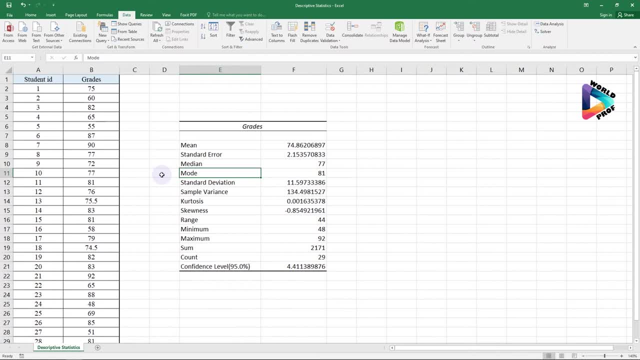 don't be surprised, because in some data sets you don't have any mode. I have already explained about the standard deviation. So, as you know, standard deviation basically tells us how each data point is far from the mean. Okay, so this is the average distance of data points. Okay from the mean. Then we have 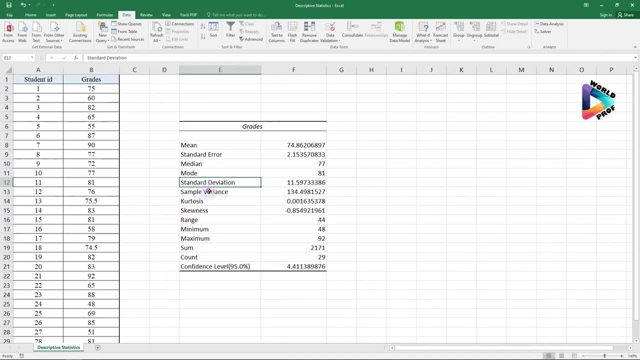 the sample variance. So sample variance and the standard deviation are also similar, but depending on what you want to do, they have different purposes. One thing you need to understand is: standard deviation gives you a value which is in the same units as the mean, But variance okay, it's the. 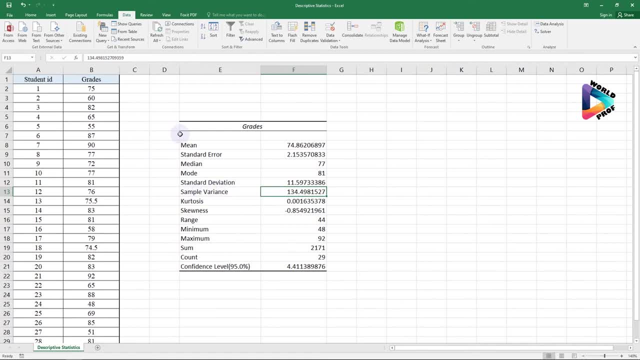 difference is that it's a squared. It's not the same unit as the mean. So if you take the square root of variance, you find the standard deviation. Okay. so the thing is that here, when we want to find the distance of each data point from the mean, Sometimes we get negative numbers. So in 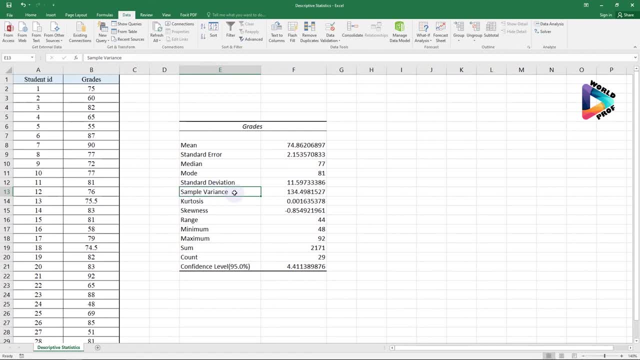 the formula of variance. Excel automatically calculates the variance. It's gonna square all those negative values to transform them into positive values, And sometimes you're getting a big number, which is not realistic. So here, if we take the square root of variance, we get the standard deviation. 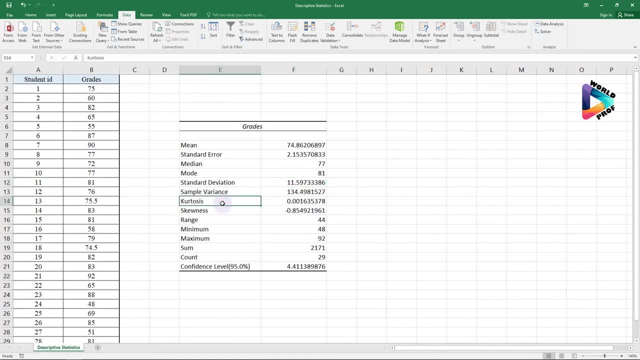 deviation. Then we have the kurtosis. So basically, kurtosis is about the tails of our distribution. It basically identifies if the tails of this distribution contains extreme values. So if the number is greater than one, it means that the distribution is too peaked. So that's about kurtosis. Then we have 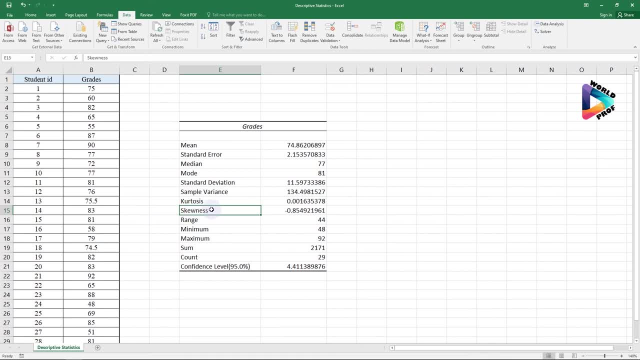 the skewness. So here that's about again the distribution of our data. But when you visualize your data you want to see whether the data is positively skewed or negatively skewed. So if the number of skewness is higher than one, okay, or than minus 1, it basically tells you that you know the data is skewed and you know. 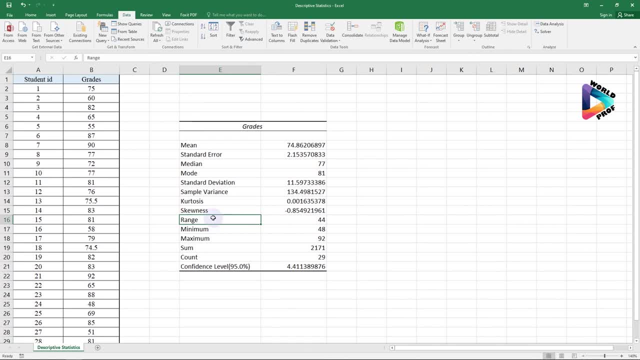 you have a skewed distribution. then you have the range in your data set, you have the minimum value. so here it tells us that the minimum grade is 48. the maximum grade is 92. it calculates the sum of all grades as well, so here you have the sum.